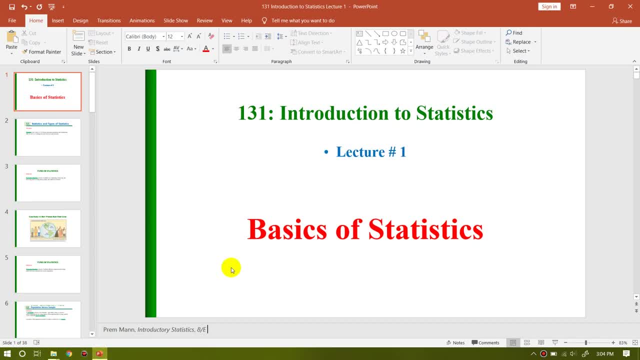 hello and welcome. this is video number 131 and I am starting another series of lectures on introduction to statistics. this is lecture number one and in this lecture I am going to focus on basics of statistics and I dedicate this video to Prem Mann, and this is based on introductory. 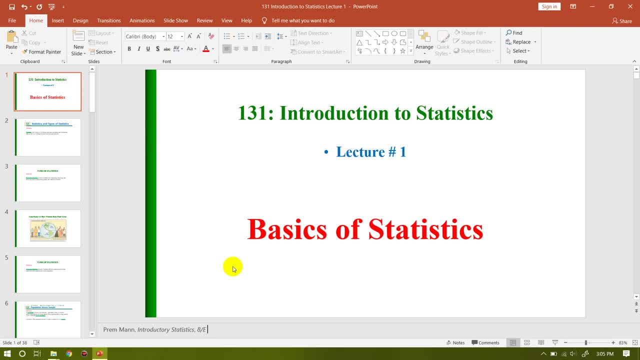 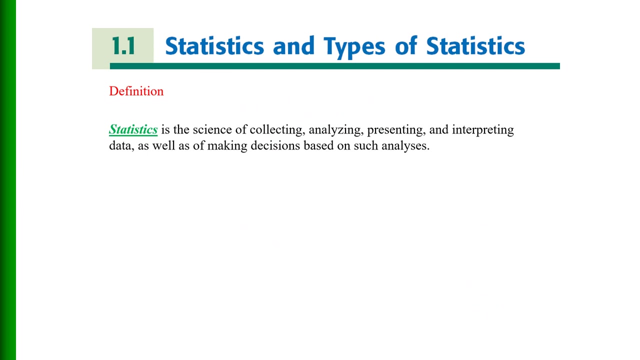 statistics edition. so this whole presentation is based on Prem Mann book introductory statistics. so this is his work and I dedicate this to Prem Mann. so, ladies and gentlemen, let me start with the definition of statistics. statistics is the science of collecting, analyzing, presenting and interpreting data, as well as of making decisions based on such analysis. there are 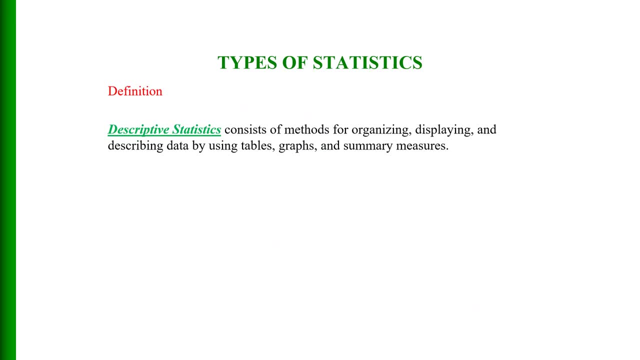 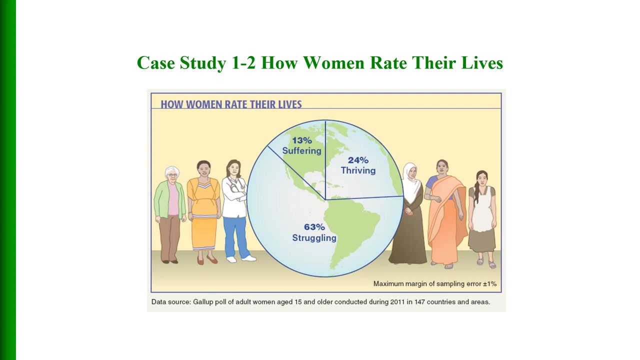 different types of statistics. the first one is descriptive statistics, and descriptive statistics consists of methods for organizing, displaying and describing data by using tables, graphs and summary measures. this is a kind of case study: how women rate their lives. so this is a kind of descriptive statistics, and here you see pi diagram and in which you see 63 percent of 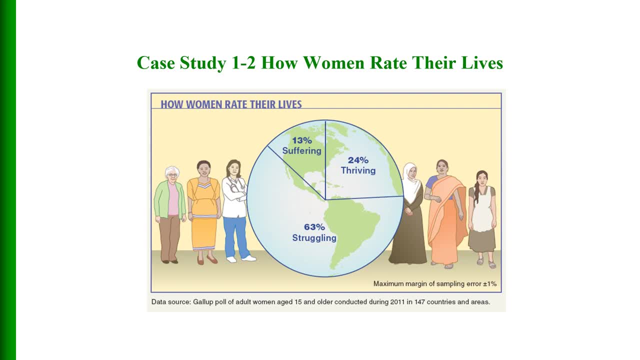 the women reported that they are struggling, 24 percent of them reported thriving and some 13 percent reported that they are suffering. so this is a kind of descriptive statistics and this is a pi diagram and the. there are three types of answers to this question and the answers are in percentages. 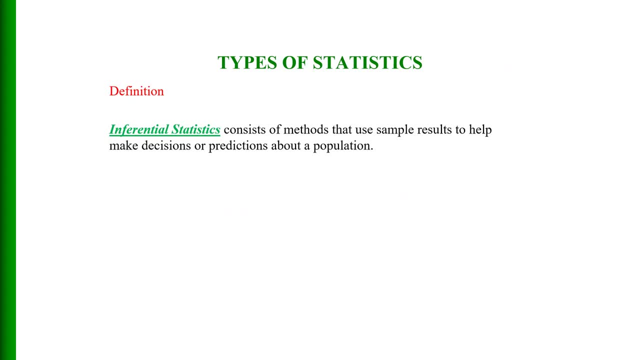 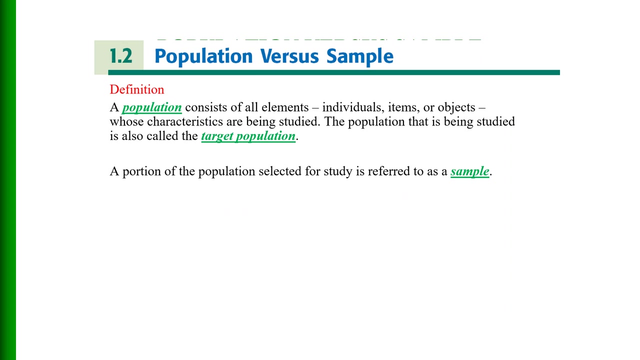 another type of statistics is inferential statistics. inferential statistics consist of methods which use sample results to help make decisions or predictions about a population. there is a difference between population and sample. a population consists of all elements, that is, individual's items or objects whose characteristics are being studied. the population that is being 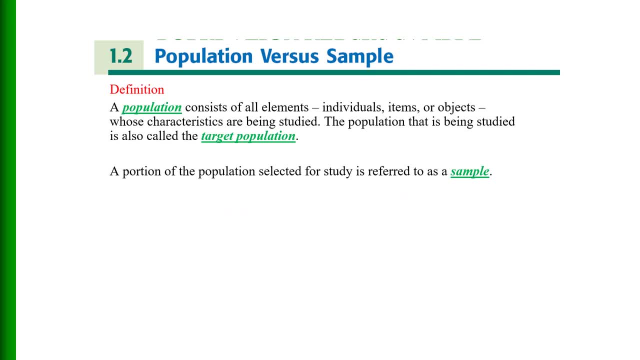 studied is also called target population. on the other hand, a portion of the population which is selected for study is referred to as a sample. so a sample is a subset of a population, it's from population and it is a portion of the population which is selected for study. here is an example. 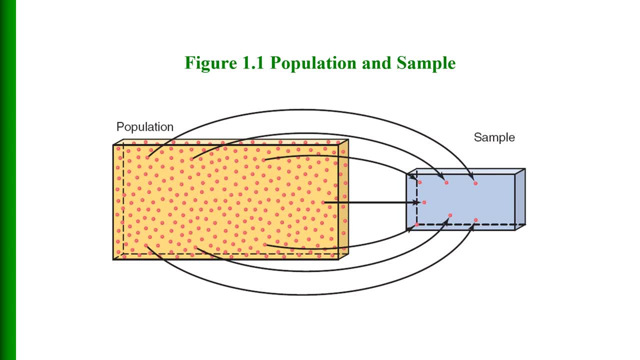 this figure portrays the difference between population and sample. on the left hand side, you see, this is population and it consists of all elements under consideration. so all these red circles are dots, are the elements, are items, are objects which are contained in this population. and on the right hand, 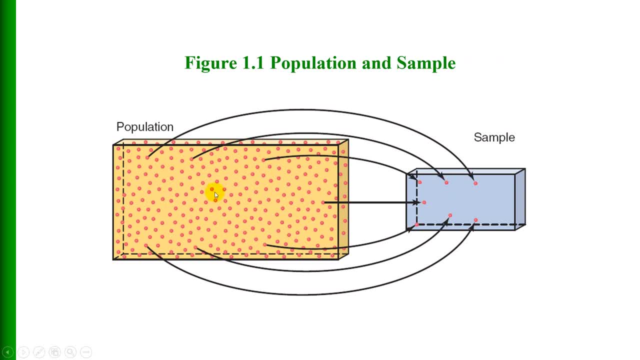 side. you see, this is a portion of this whole population. so this is a sample. so a sample is a small portion of the population. so you see, uh, population contains a large number of elements, whereas this sample contains only one, two, three, four, five, six, seven elements. so it's a part of the population. a survey which 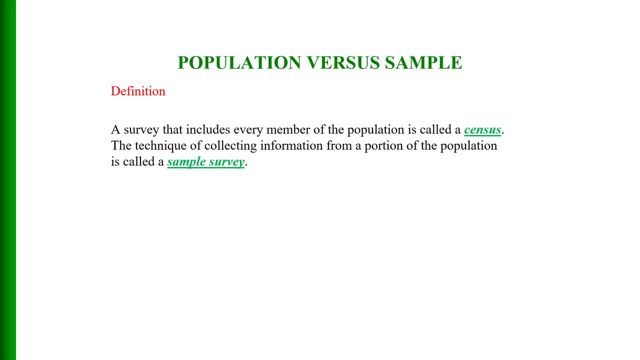 includes every member of the population is called a census. the technique of collecting information from a portion of the population is called a sample survey. so one is census and one is sample survey. in census we include each and every member of the population, whereas sometimes we select a sample from the 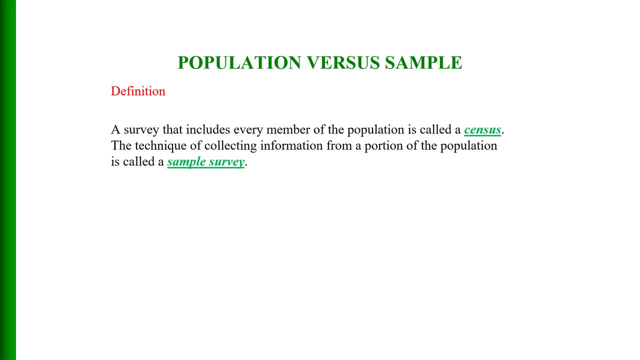 population and then we make a survey and that survey is called is a sample survey. a sample that represents the characteristics of the population as closely as possible is called a representative sample, and this is very much needed for your research. if you select a sample from the population, it 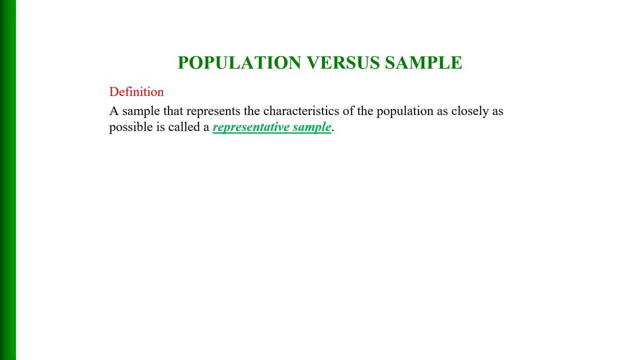 must be representative. if it is not representative of the population, then your results may not be reliable. a sample drawn in such a way that each of the elements of the population has a chance of being selected is called a random sample. if L samples of the same size selected from a population have the same chance of being selected, we call it. 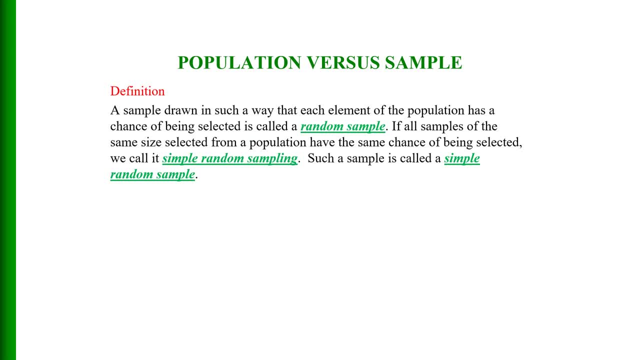 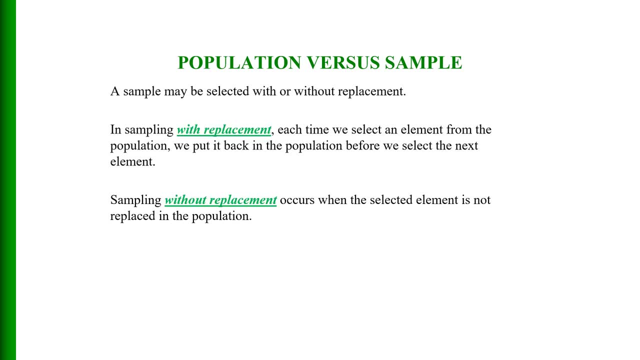 simple random sampling. such a sample is called a simple random sample. a sample may be selected with or without replacement in sampling. in sampling with replacement, each time we select an element from the population we put it back in the population before we select the next element. so this means we have sampling with replacement, sampling without. 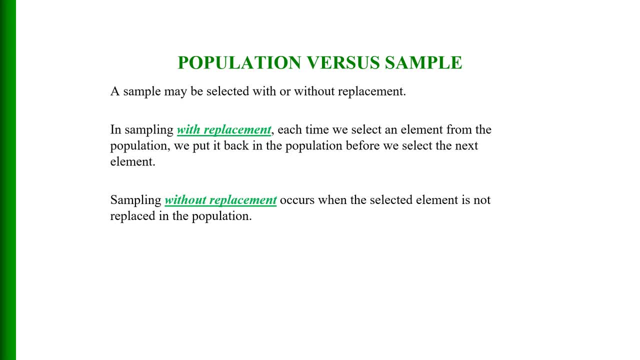 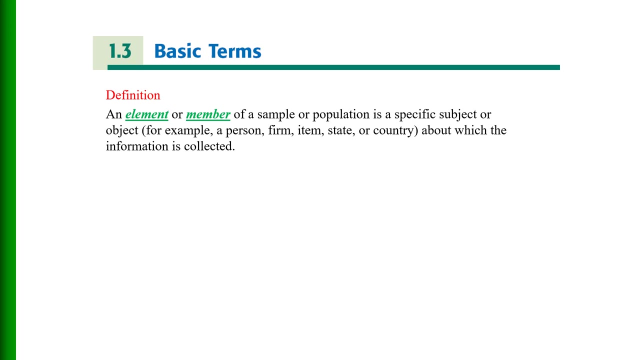 replacement occurs with the following agencies: when the selected sample is not replaced in the population, we don't put it back in the population before we select the next element. an element or member of a sample or population is a specific subject or object, for example, a person, a form, an item, a state or a country about which the information is collected. 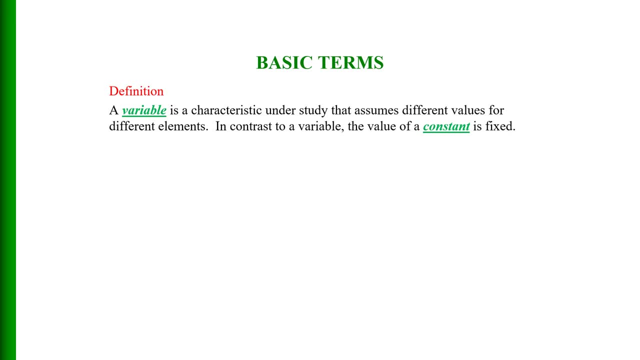 then we have variable. a variable is a characteristic under study that assumes different values for different elements. in contrast to a variable, the value of a constant is fixed. the value of a variable for an element is called an observation or measurement. a data set is a collection of observations on one or more variables. here is an example. 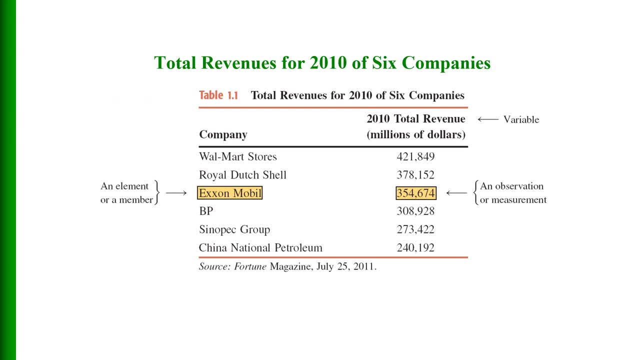 in this table. this is the total revenue for 2010 of six companies. now here are the six companies: walmart stores, royal dutch shell, exxon mobile, bp, sinopec group, china national petroleum, and here are the total revenue. these are in millions of dollars, so this particular value is an observation or measurement. 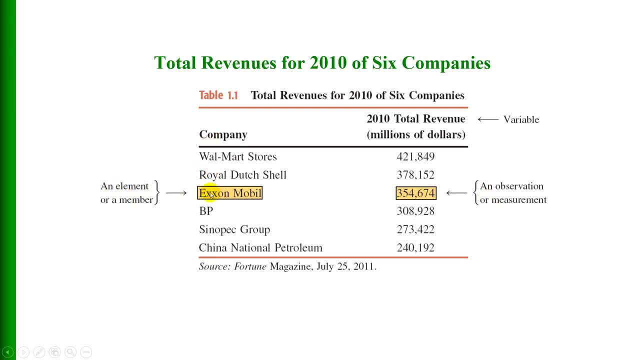 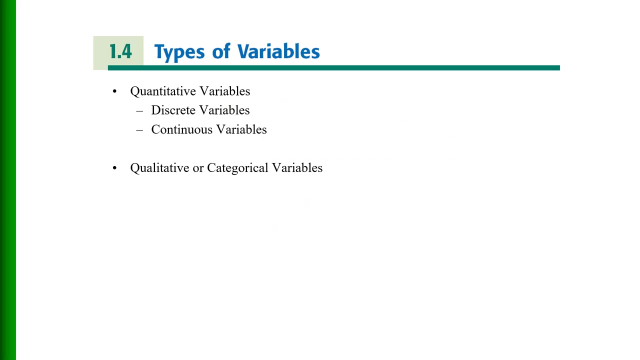 and this is in element- are a member of these companies and this is the total revenue. this is a variable. so you see, total revenue varies from company to company. so this is how observation element or a variable can be distinguished from each other. then there are types of variables. variables may be quantitative. 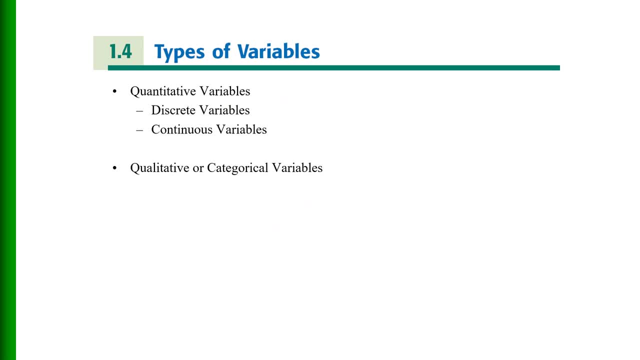 or qualitative. quantitative variable may be discrete or continuous. qualitative variables are also called categorical variables. quantitative variables: a variable that can be measured numerically is called a quantitative variable. the data collected on a quantitative variables are called quantitative data. a variable whose values are countable is called a discrete variable, in other words, a discrete. 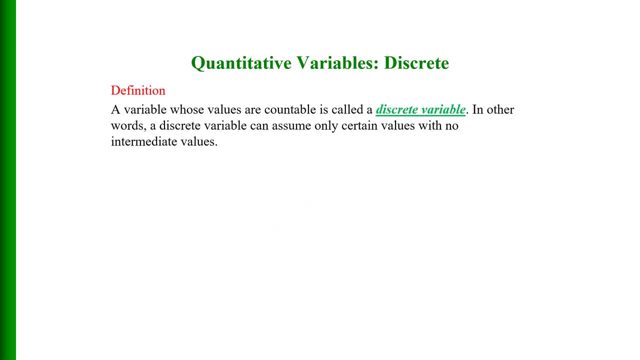 variable can assume only certain values with no known data that are considered countable, only certain values with no intermediate values, say, for example, age, consumption, income, height, weight and so on. these are discrete variables, but these are quantitative variables also. then we have continuous variable, a variable that can assume any numerical value or a certain. 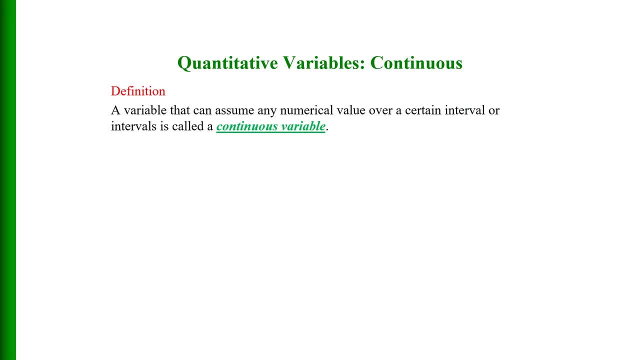 interval or intervals is called a continuous variable. now, age and weight or speed of a car are types of a continuous variable. a variable that cannot assume a numerical value but can be classified into two or more non-numeric categories is called qualitative or categorical variable. for example: male, female, yes, no. 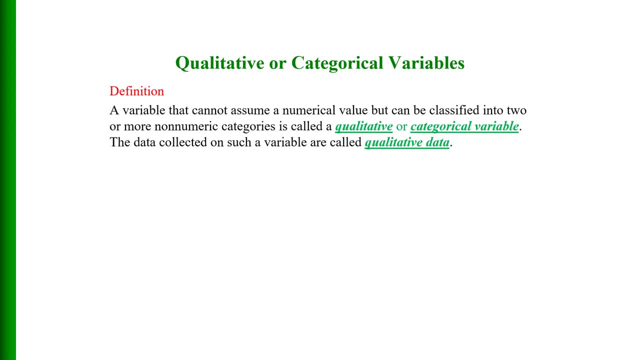 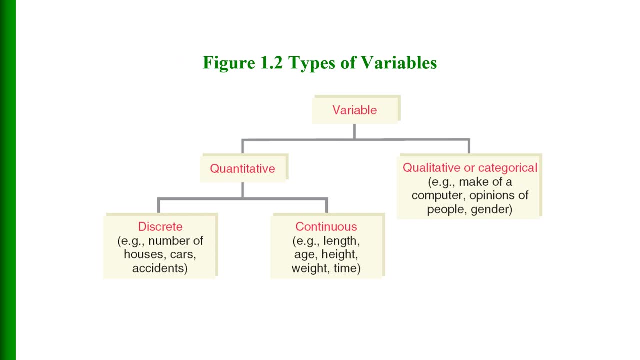 black, white, muslim, non-muslim and so on. the data collected on such variable are called qualitative data. here are the types of variables. with the help of this figure you can see. here is the variable, here is the quantitative variable, and then within quantitative variable we see discrete, for example, number of houses, cars, accidents, number of deaths. 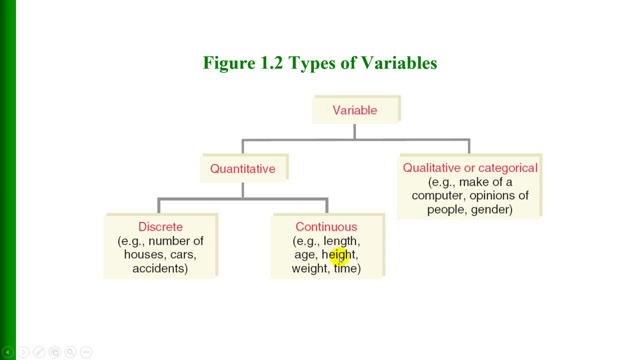 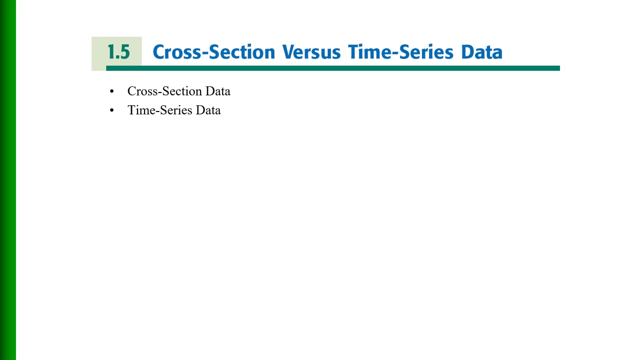 continuous length, age, height, weight and time. these are continuous variable, and here you see qualitative or quantitative categorical variables. for example, make of a computer, opinions of people, gender and so on. uh data may be cross-section or time series. it can also be panel data. so here this is just for the beginners. so we just differentiate between cross-section data. 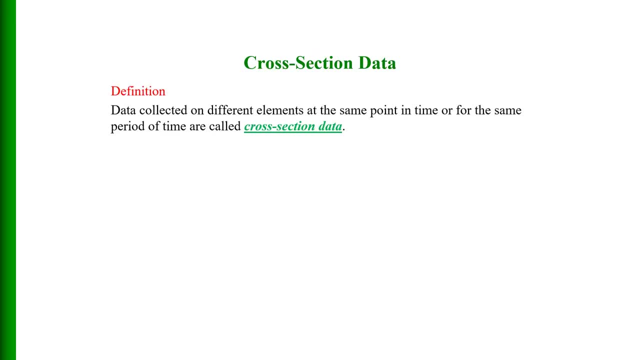 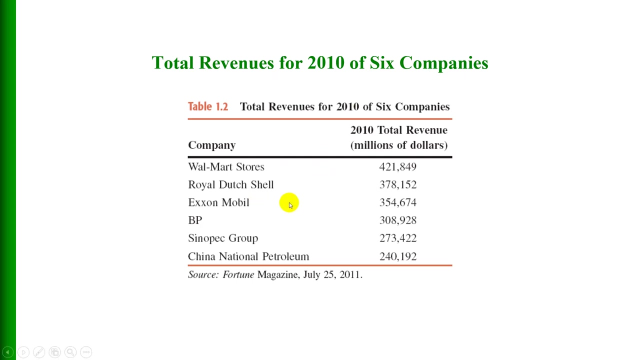 and time series data. data collected on different elements at same point in time or for the same period of time are called cross-section data. for example, this is a an example of cross-section data. this is total revenue in millions of dollars and these are companies, and this data is for, say, 2010. so this is cross-section data for the same period of time. 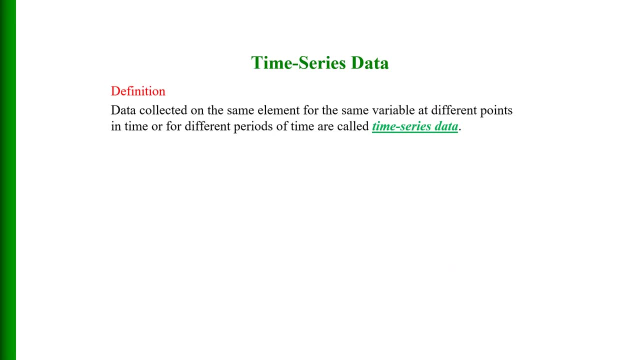 then there is time series data. data collected on the same element for the same variable at different points in time are for different periods of time, are called time series data. for example, data on gnp data, on national income data, on exports data and export data on investment, consumption, saving and so. 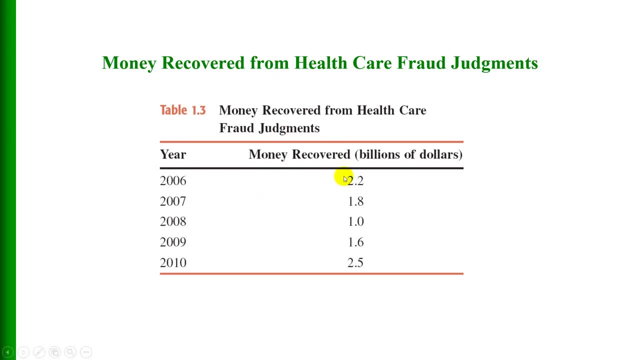 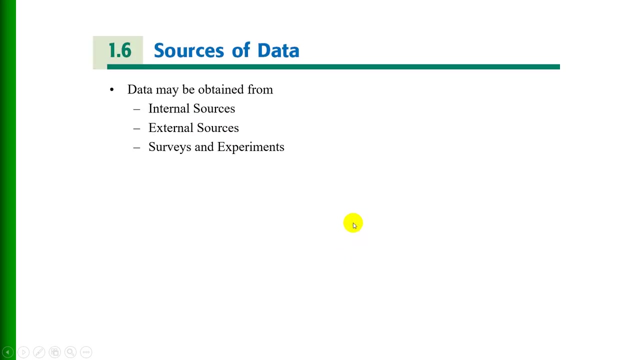 on. and here is an example of uh: money recovered from healthcare for fraud judgment. so this data is on the same variable, uh, over a period of time that is 2006, 2007, 2008 till 2010, and these are billions of dollars recovered. so this is a kind of time series data. uh data could also be panel. 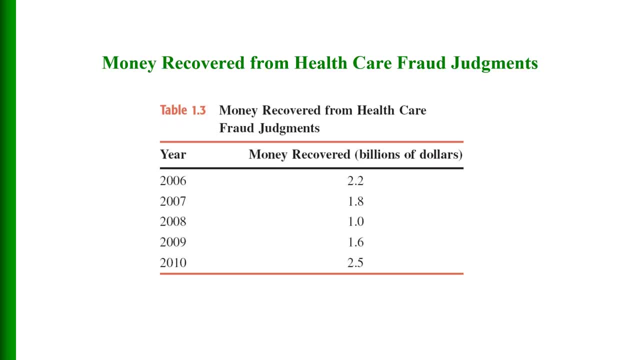 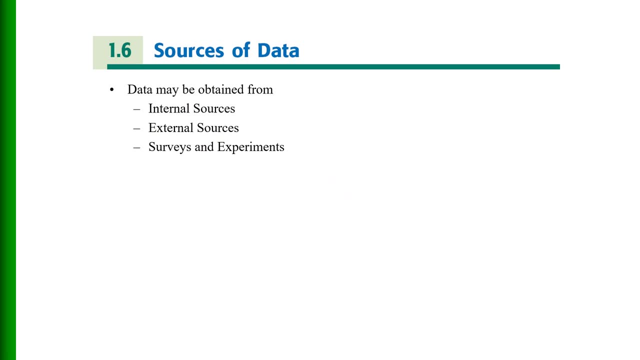 data when we combine the cross-section data and the time series data, so this is a kind of time series data. uh data could also be panel data. when we combine cross-section and time series data, we get panel data. these are sources of data. data may be obtained. 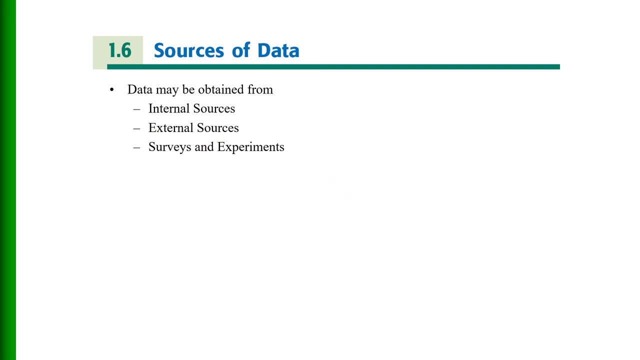 from internal sources or external sources. we may also call them primary sources or secondary sources. primary sources are those when we collect data for the first time, and secondary sources are those which are in published books or reports, surveys and so on. we also obtain data from surveys and experiments. 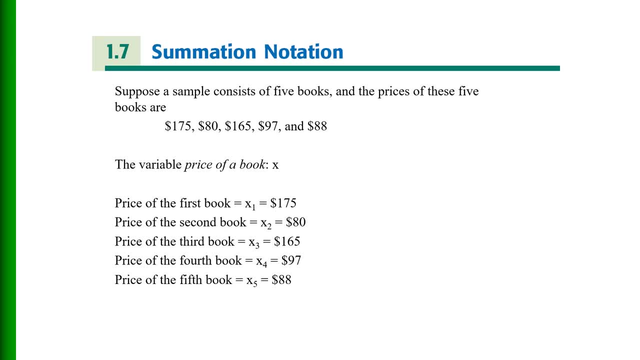 here are some notations, and in statistics and mathematics we use this notation more often and that is summation notation. suppose a sample consists of five books and the prices of these books are as follows: book number one costs 175 dollars. price of the second book is 80 dollars. 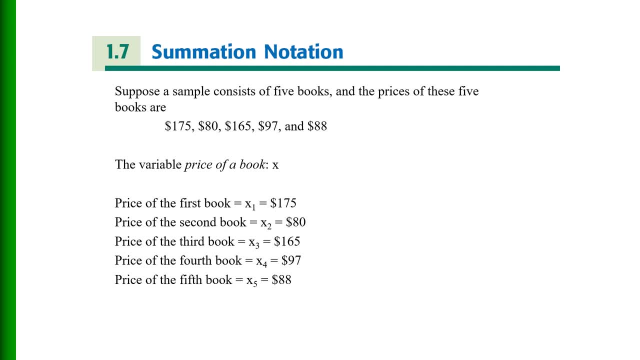 price of the third book is 165 dollars, price of fourth book is 97 dollars and price of the fifth book is 88 dollars. so the variable price of a book is x. let us suppose x stands for price of a book. so this is a variable. it varies from book to book. so price of the first book is x1, price of the second. 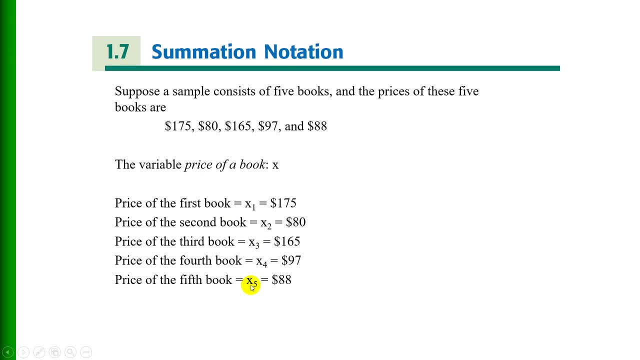 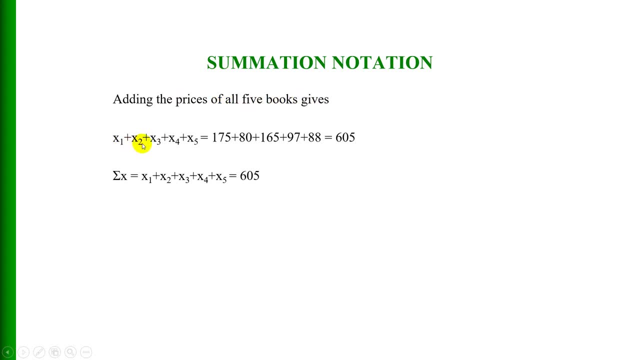 book is x2 up to x5, so this is equal to bob goldwell. you will get for the first book x1, required by a constant advantage over x1, and then x2. so adding these prices of all the five books gives x 1 plus x2. 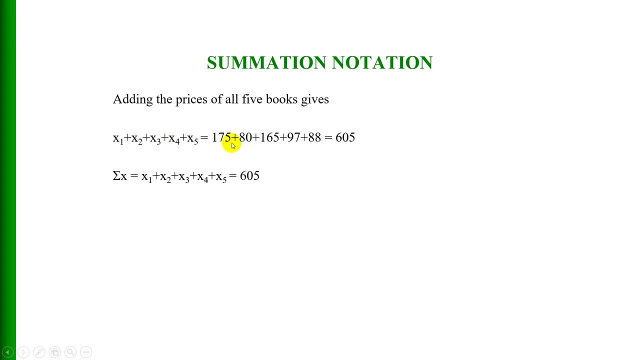 plus x, 3 plus x, 4 plus x, y, 0, and that is equal to 175 plus 80 plus 165 plus 97 plus 88, and the sum is equal to 605. so we can write that mathematically: summation x- i, where i varies from one to five, and that is equal to six hundred and five. so 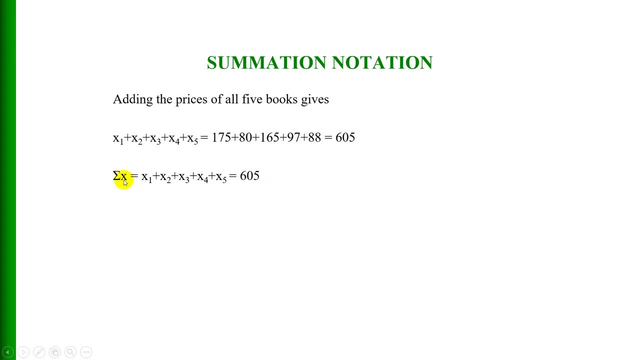 this is the summation notation. so this is the bottom page in which, if youныеxtomex and summation notation means we add all prices of the five books. here is an example: annual salaries in thousands of dollars of four workers are 75,000, 90,000, 125,000 and 61,000 respectively. 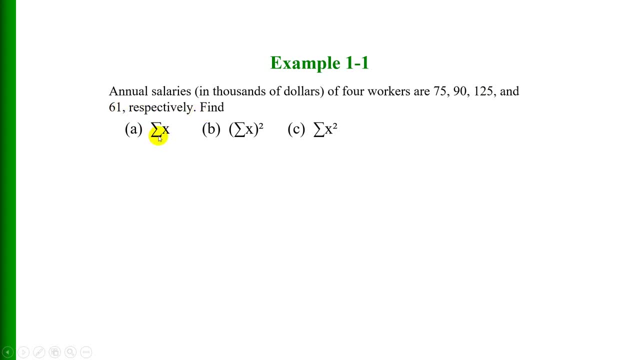 then find number one: summation x, b. summation x whole square, c, summation x, square. so here is the solution: summation x is equal to x1 plus x2 plus x3 plus x4. where x1 is 75, x2 is 90. 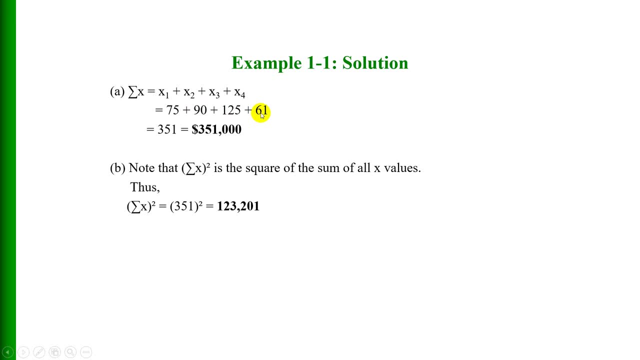 x3 is 125 and x4 is 61 and the sum is equal to 351. so we can write that in 351,000 dollars. the second question was summation: x whole square. so that is the square of the sum of all x values. so we will square this so summation. 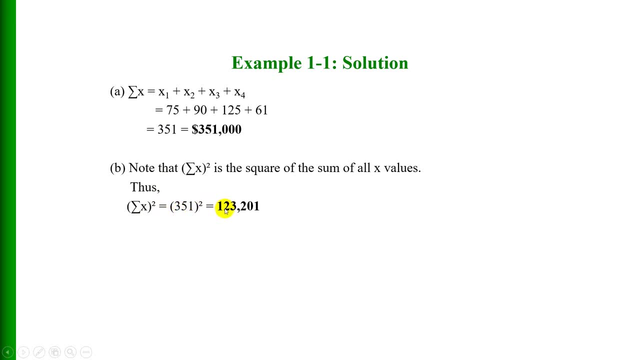 x whole square is equal to 351 square and that is equal to 123,201. so this is: summation x is equal to 351. summation x whole square is equal to 123,201. the c part of the question is the expression: summation x square is the sum of the squares of x values. to calculate summation x. 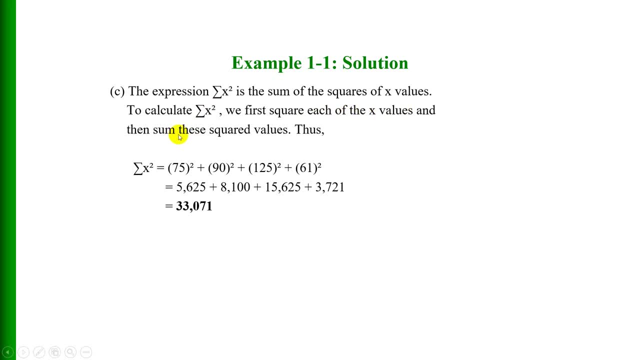 square. we first square each of the x values and then sum these squared values. for example, we can write summation: x square is equal to 75 squares plus 90 square plus 122 square plus 61 square, and the 75 square is equal to 5625. 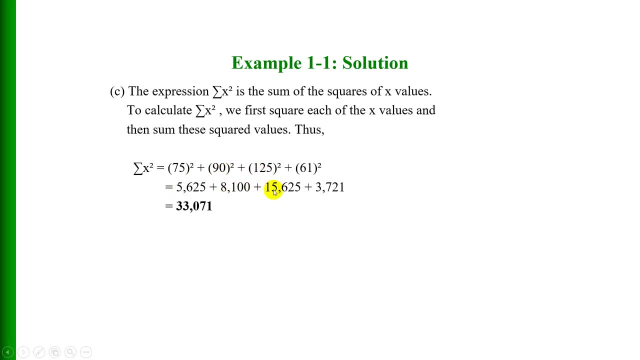 is equal to 8100, and this is equal to 15625, and this square is equal to 3721 and if we add up all these we get 33,071. so there is difference between summation x- square and summation x whole square. 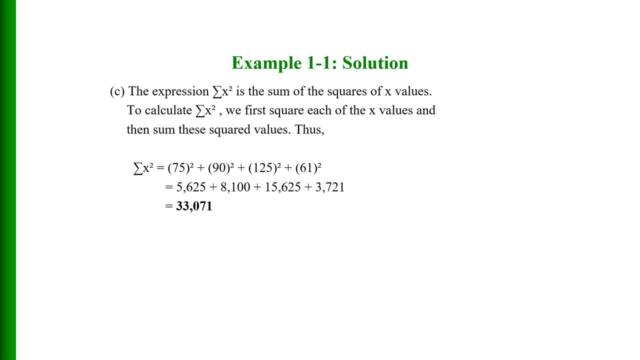 because summation x- square is equal to 33,071, whereas summation x whole square is equal to 123,201. so you must be very careful about calculating these values. there is a big difference between summation x- whole square and summation x square. here is the example. 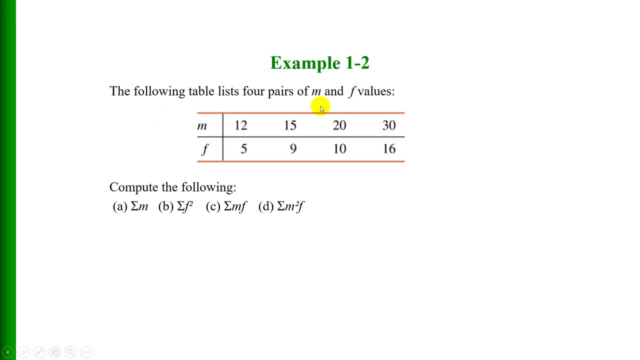 the following table lists four pairs of m and f values. m is a 12, 15, 20, 30 and f is a 5, 9, 10 and 16. so the question is how to compute the following summation: m, sum of m. these values. 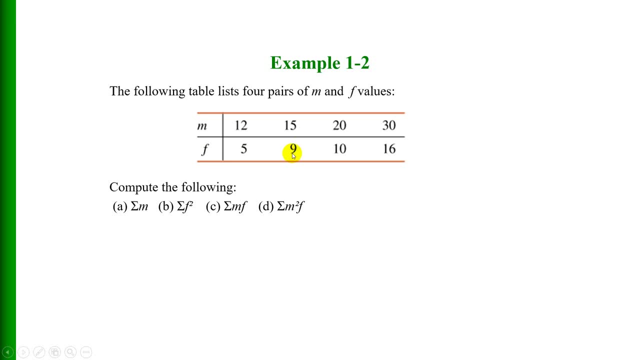 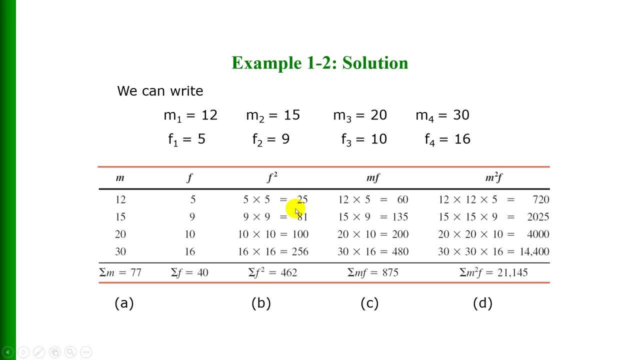 then sum of f- square, and then summation m- f and summation m square- f. so we can write: m 1 is equal to 12, m 2 is equal to 15, m 3 is equal to 20, m 4 is equal to 30. 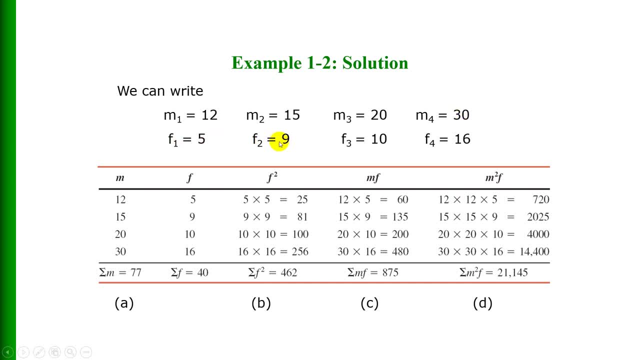 5, 7. f 1 is equal to 5, f 2 is equal to 9, f 3 is equal to 10, excuse me, f 4 is equal to 16. so the m values are there. so if we sum these values, we get summation m and that is equal to the sum of. 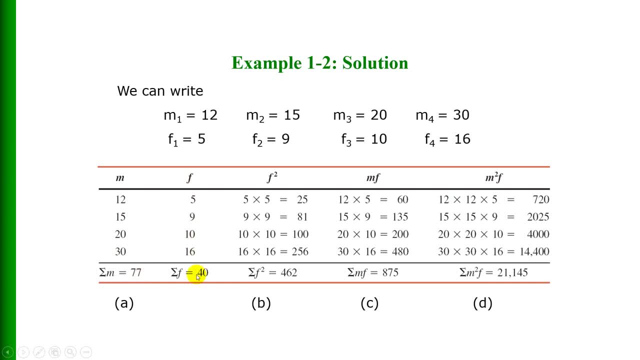 these four values is equal to 77 and this is the sum of f. that is equal to 40, and f square is: this: is f. so multiplied by 5, then 9, multiplied by 9, then 10 multiplied by 10, then 16 multiplied by 16.. 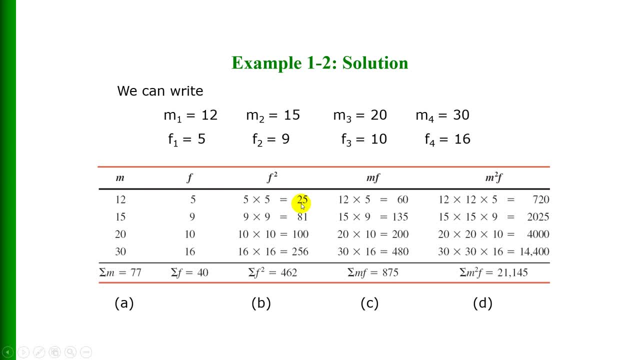 So we get these values: 5 into 5 is equal to 25, 9 square is equal to 81,, 10 square is equal to 100 and 16 square is equal to 256.. So if we sum up these values, then we get: 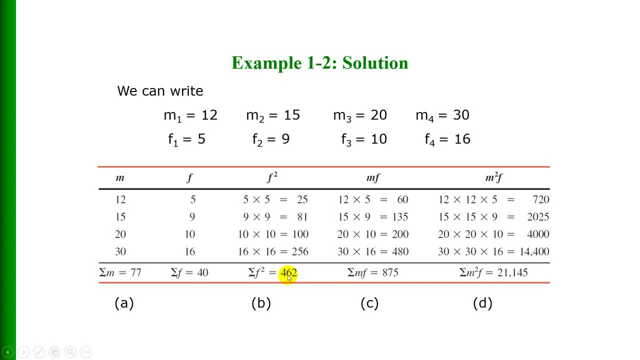 summation f square, and that is equal to 465.. Then we come to mf. What we do? We multiply m with f, So we have: 12- 5s are equal to 60, 15- 9s are equal to 135, 20- 10s are equal to 200 and 30- 16s are. 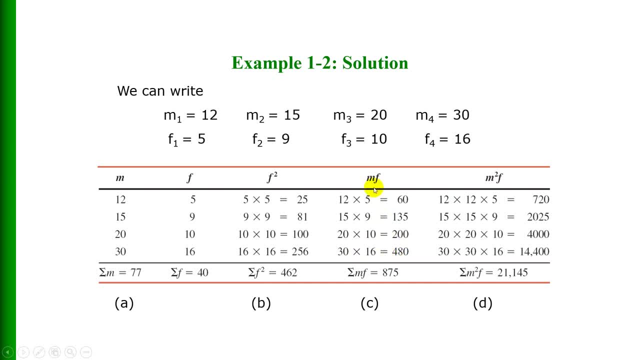 equal to 480, and if we sum up these then we get summation mf and that is equal to 875.. Then we come to m square f, Since we need to calculate summation m square f, so first we need to have m square. Here is m, So first we square this, So 12 multiplied by 12, and then f. 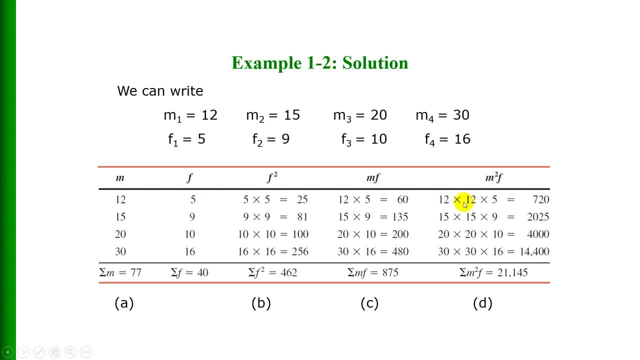 is equal to 5.. So 12 into 12 into 5 is equal to 720.. Then 15 into 15 into 9 is equal to 2025.. Then 20 into 20 into 10 is equal to 4000, and 30 into 60 is equal to 14400.. And if we add up all, 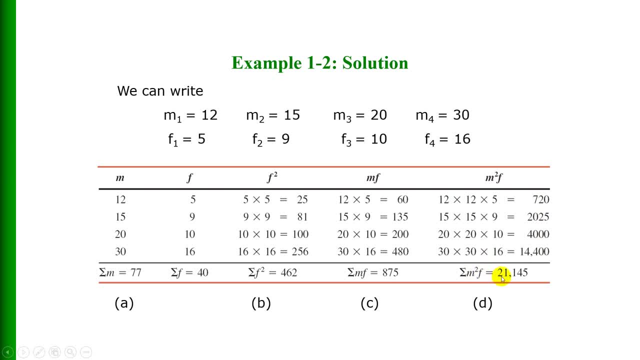 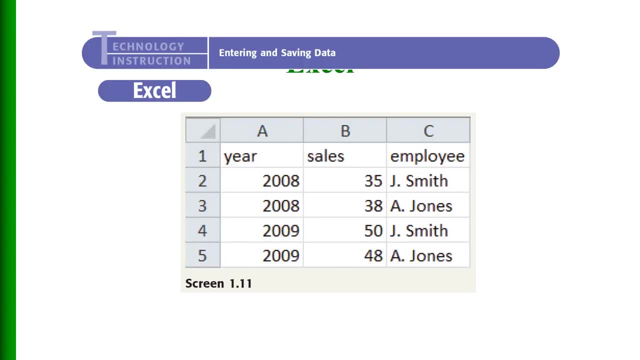 these values, then we get summation m square f and that is equal to 21145.. These are small examples And this is how we can enter and save data in Excel. Usually we see in the first we have number, of observations, numbers, and then we have a, b, c columns so we can write here and then. 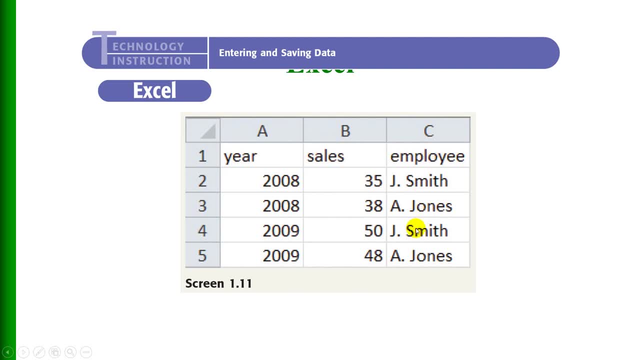 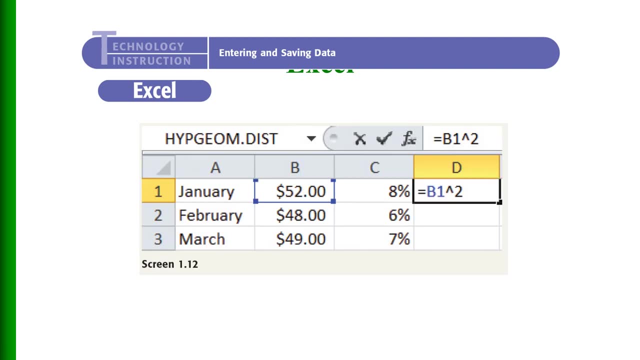 we can write sales and we can write employee name. so this is how we enter our put data in excel. again, this is january, february, march, and these are some numerical values- dollars and these are some percentages. and this is a if. for example, if you want to calculate the square, 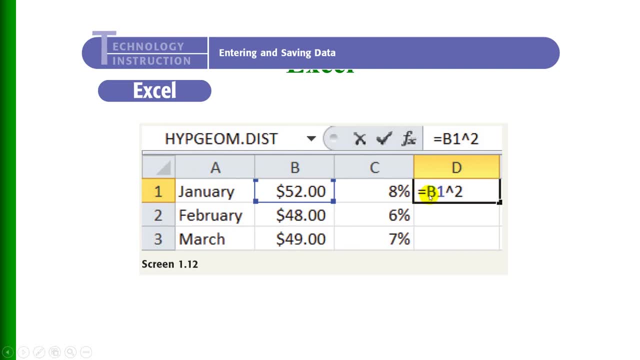 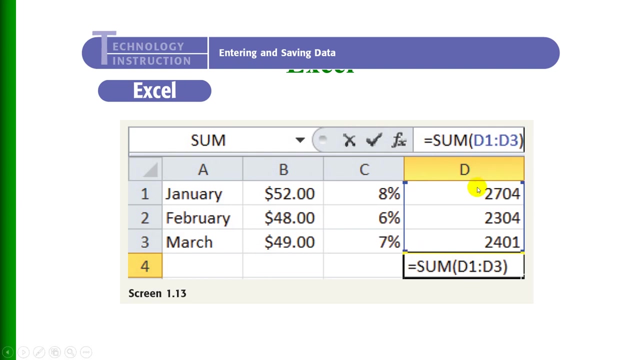 of this. then you write like this: equal sign v1, hat 2. so if you press this, then it will calculate the square of this. similarly here also: if you copy, then it will calculate square for these values also. uh, yes, and here in this you see, this is the formula, the. 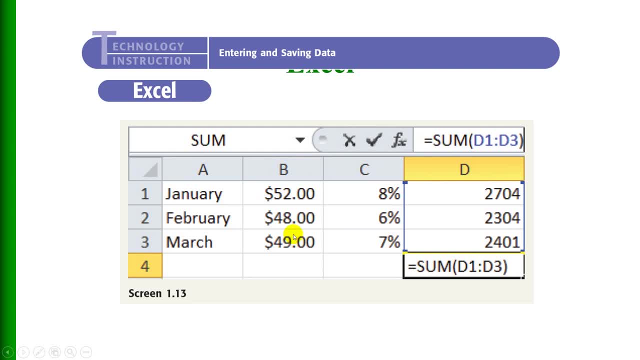 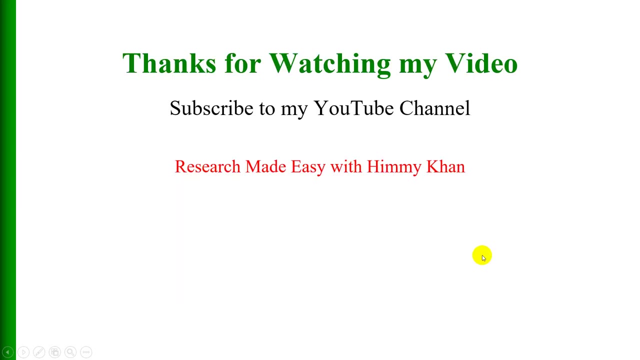 the square of this is equal to this, and the square of this is equal to this, square of this is equal to this. so if you want to sum up all these, then here you will get the addition of all these, maybe in the next. so, ladies and gentlemen, this was a brief introduction to 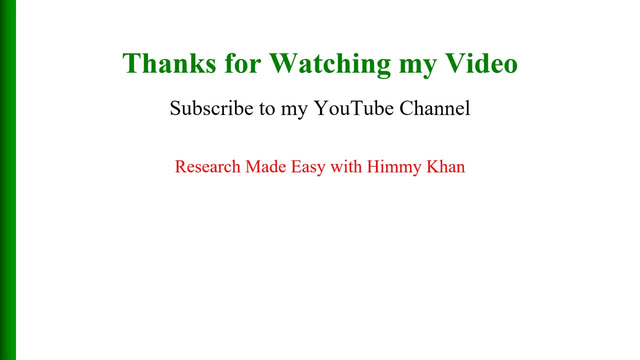 various uh concepts, topics in introduction to economics. this is. this video is meant only for the beginners. thank you for watching. if you like the video, kindly subscribe to the channel and share it with your friends and with your colleagues so that it can lead to maximum possible number of people. and kindly do not forget to click on bell icon so that you can get the new.